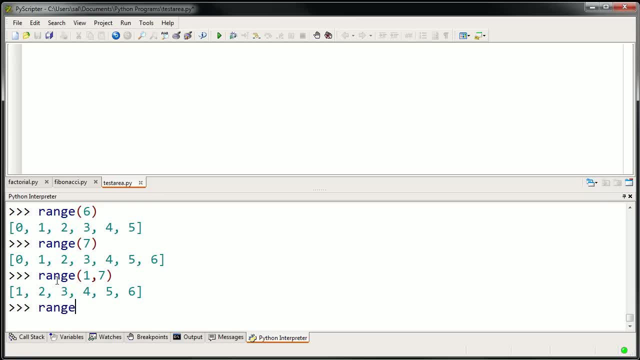 environments, these IDEs, this PyScripter that I'm running is that when I type in a function that it recognizes, it actually will tell me a little bit something about that function, in case you forget it. So I don't know if you can read this here. 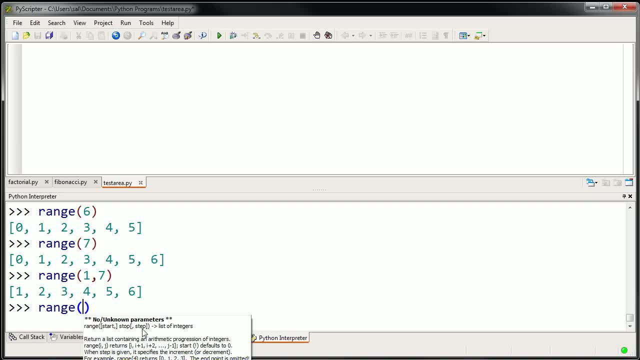 but it says: range, start, stop, step. So you can also, if you want, tell it how much to increment. So right now the default is to increment by 1 each time, But it says: hey, I could tell you. 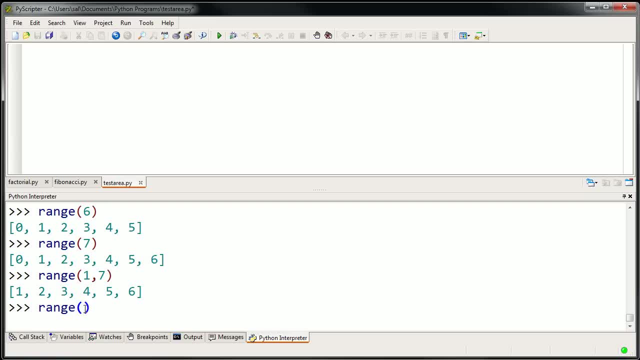 to increment by a different number. So let's say you have a range, say you start at 0. You want to go up to 8, and I want to go up by 2 instead of 1.. So then I went 0,, 2,, 4,, 6, and I should have said it more. 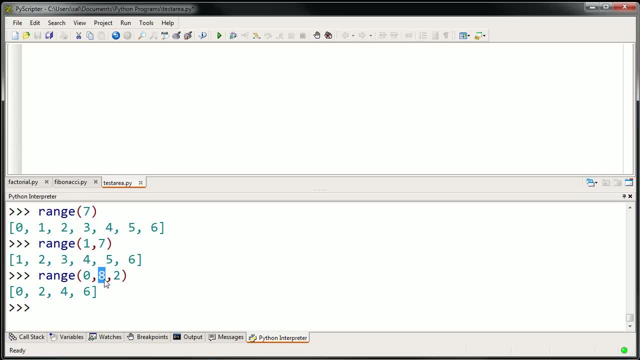 precisely up to, but not including 8. The upper part of the range: you don't include it, So it goes up to that and it increments it by 2. So you could do it like that, Or you could even so. maybe you want. 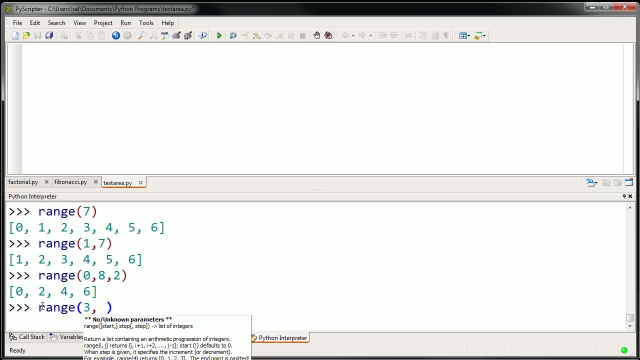 to start at. maybe you want to start at 3, and you want to go up to, but not including. I don't know. let me do up to, but not including 31.. And you want to go up by steps of 3.. 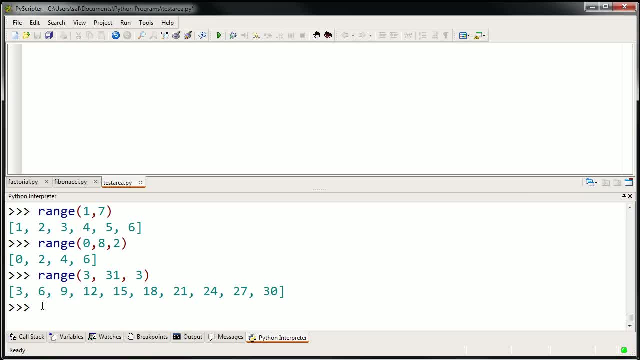 So there you go. It went up to step by 3, up to, but not including 31.. So it can generate a whole bunch of lists, And the reason why this is useful is because we can use these inside of loops, And so the first type of loop I'm 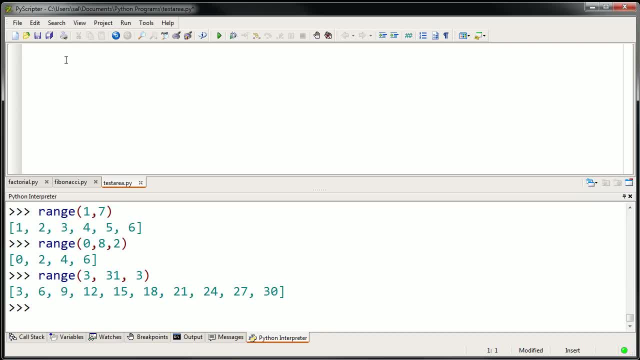 going to introduce you to is a for loop. So this was the interpreter down here. Here I'm going to actual write a program. So this program is really just to show you what a for loop does. So I could say: for i and i is this variable, that's. 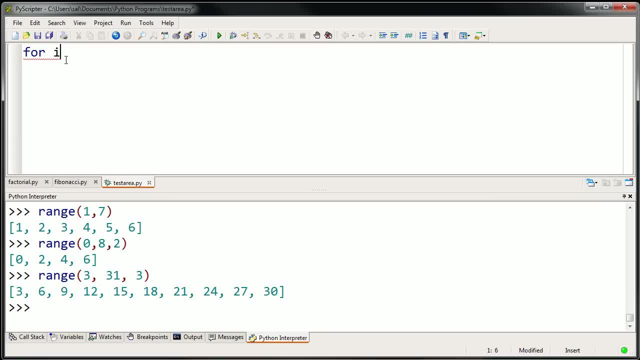 often used in for loops, in iterative loops, And iterative means you keep doing something over and over again For i in, and let me just do a simple one In range, and I'm just going to say 5, range of 5.. 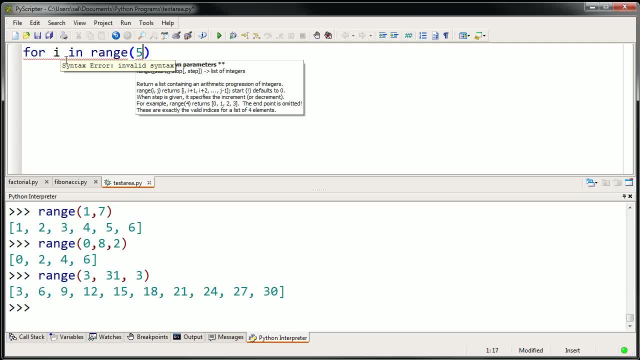 So this will generate a list: 0,, 1,, 2,, 3,, 4.. So for i in range 5.. And this colon says: now we're going to have a subclause of what to do on each of those. 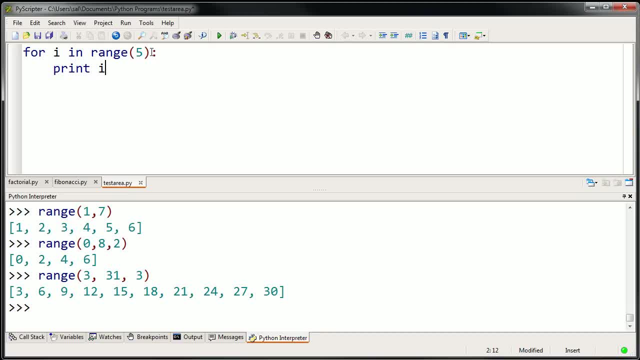 iterations. Let's just print out what i is, And so, before we even see what this is going to do, let's just think about it. It's saying: for each time we go through this loop, for each of the things in the range make i refer to them. 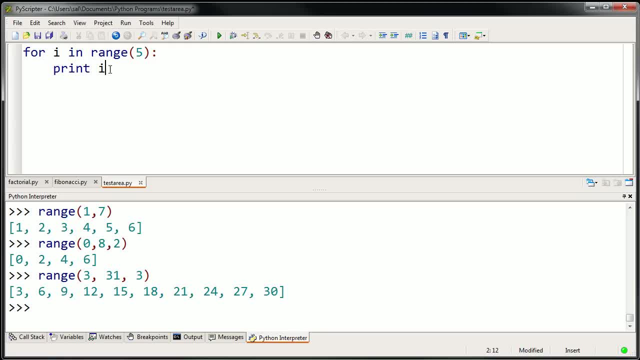 And then each of those loops is going to refer to a different one, and you want to print it out. So let's just try this out. So let me save this program and now let me run it. So there you go. What it did is it created a loop? 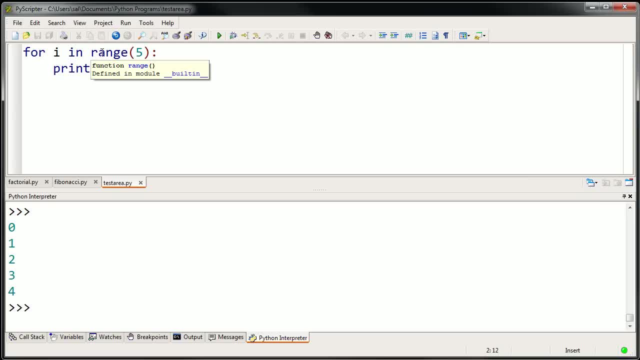 So it, Each time it goes through the loop, it assigns i to a different element in this list. As you remember, this list was 0,, 1,, 2,, 3, and 4.. And so did I say 0,, 1,, 2,, 3,, 4,, 5 before. 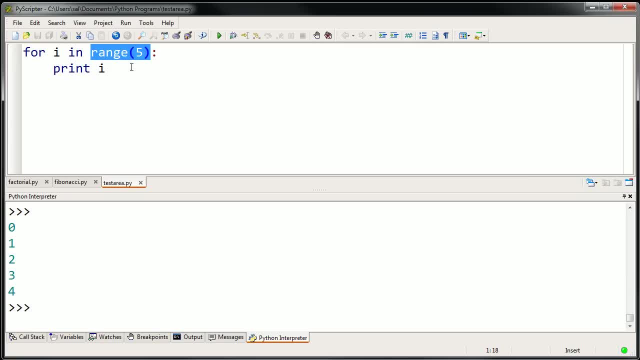 No 0,, 1,, 2,, 3,, 4, up to, but not including 5.. And so each time you go through the loop, i is, it goes through each of those items and this program really just says: print out that i. 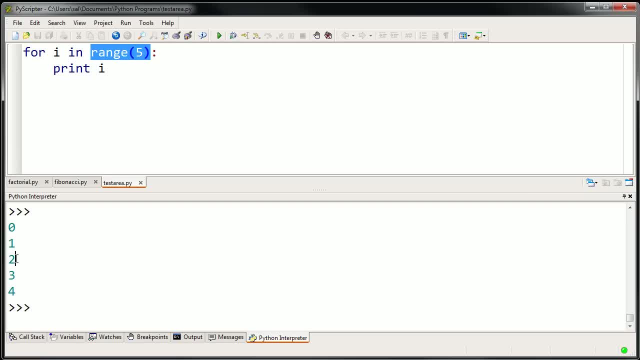 So the first time we go to the loop i is 0. So it prints it out. Then it prints out 1.. Then it prints a 2.. Then it prints a 3.. Then it prints a 4.. So it just keeps going through it that many times. 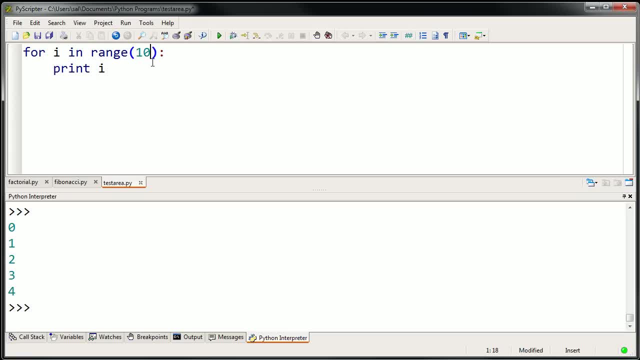 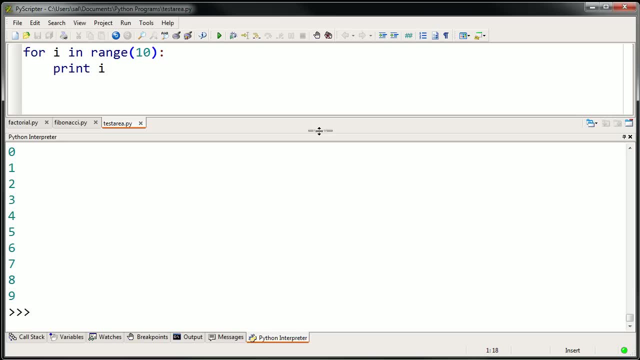 If we said this was for a range I don't know, 10.. Now let's run this program. You'll see it'll print 1 through 9.. It'll print 1 through 9.. Or I should say 0 through 9, because that's. 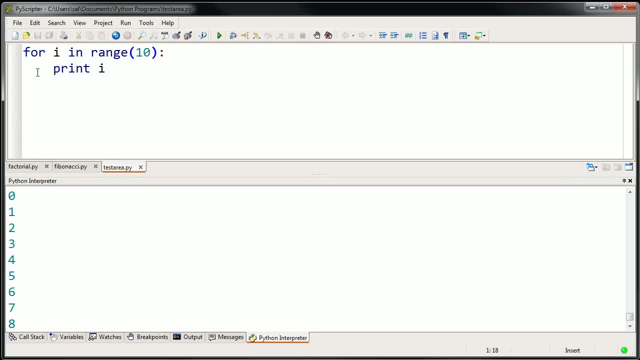 the first element in this list. But you could do more interesting things. Let's say that you wanted to take the sum of 0 through 9.. So what you could do is you could define another variable here: sum. So before I do anything, 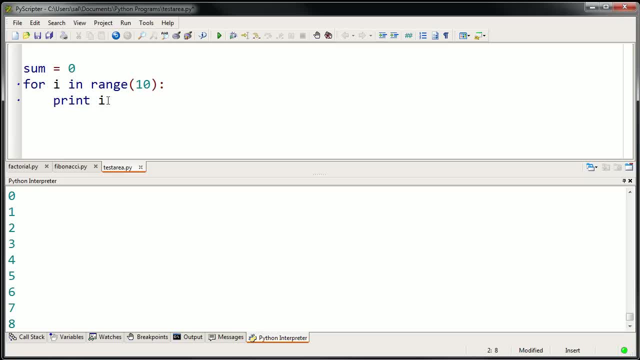 The sum is just going to be 0. And then what you could say is: each time you go through the loop, why don't you add to sum? why don't you define sum to be the previous sum plus what i is in this part of the loop? 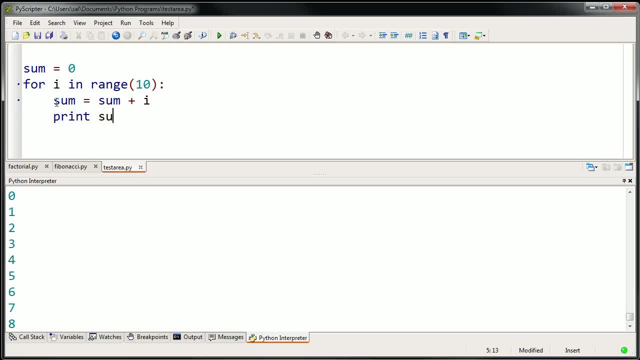 And just so that we can keep track of it, I then want to print the sum. Now, let's see what this thing does, So let's try it out. So let me save it And then let me run it. So there you go. 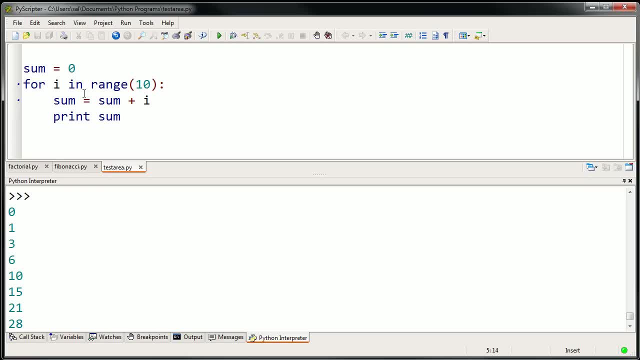 Each time we went through the loop. So the first time we went to the loop, sum is 0.. Sum is 0 and i is 0. You add them together, You print the sum, You get 0.. The next time we go through the loop, i is 1.. 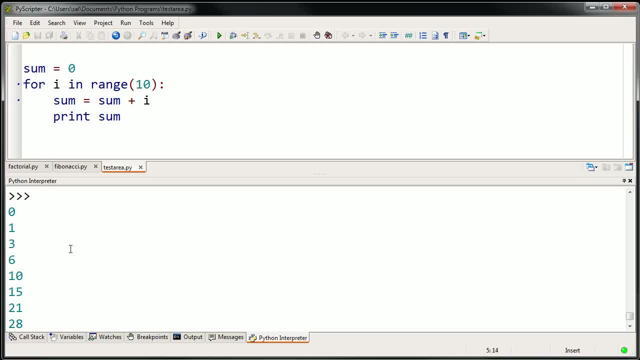 We add that to the previous sum, which was 0. Print it, You get 1.. Then the next time, through the loop, i is now going to be 2.. Add that to the previous sum: 2 plus 1, you get 3.. 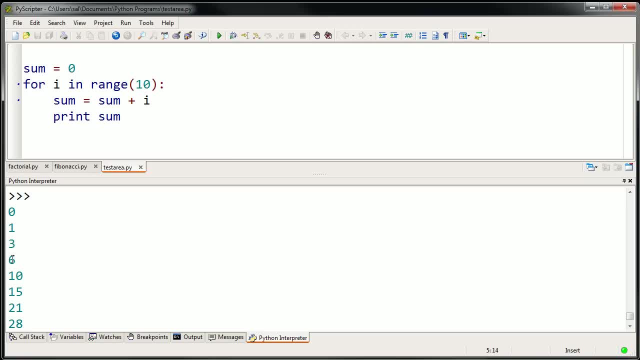 Next time through the loop, i is 3.. Add that to the previous sum, You get 6.. So the sum of all of the numbers- 0 through 9, is 45. So just that, that's actually kind of a useful program. 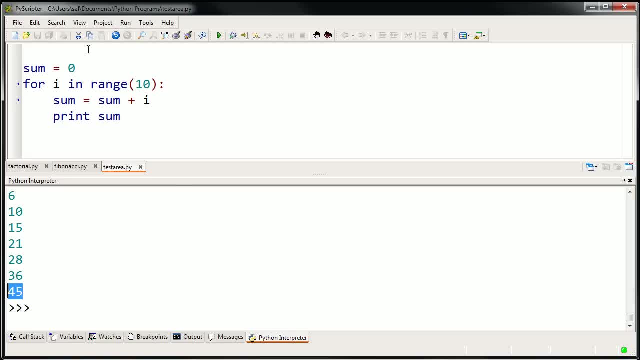 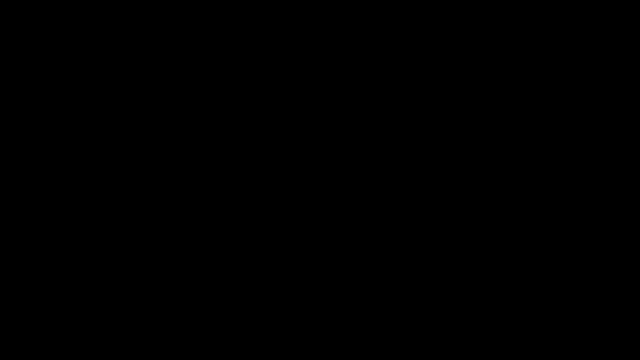 But just to make the point a little bit clearer, let me actually walk you through this on my little drawing tablet. So let me paste my code that I just wrote up here And let's just think about what this is doing. So we have a couple of variables here. 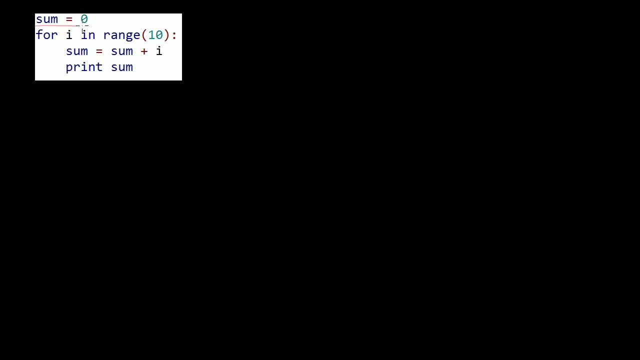 We start off with this variable sum that is set to 0. And there's two ways to visualize variables. A common way to visualize it- and this isn't necessarily wrong, This is sometimes an easier way to think about it- is to view them as buckets. 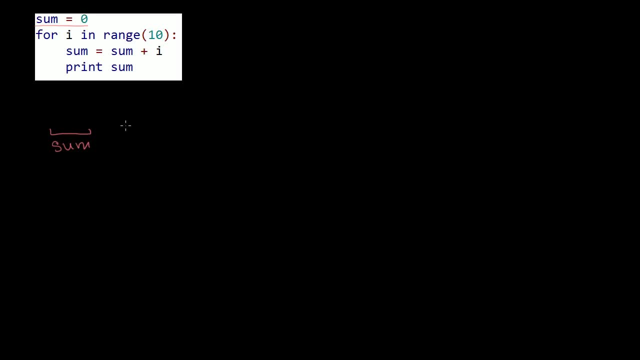 But in Python the really correct way- and you saw why that's important with lists- is to view them as referring to something. So if you view them as buckets you can kind of say: OK, from the get go. the number in the sum bucket is 0.. 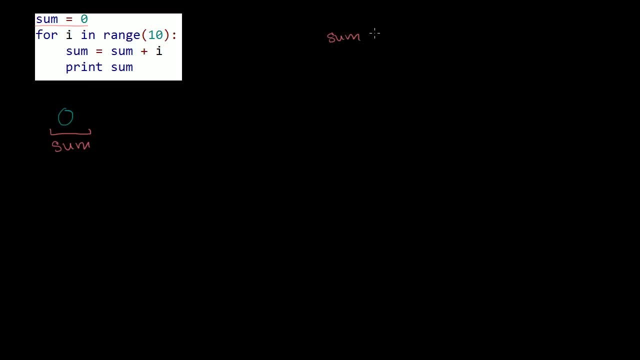 But the reality is that the variable sum is now referring to the numeric literal, the actual number 0, sitting in memory someplace. Now we enter into the for loop, And what the for loop says is: let's iteratively assign i to each of the elements in the list generated. 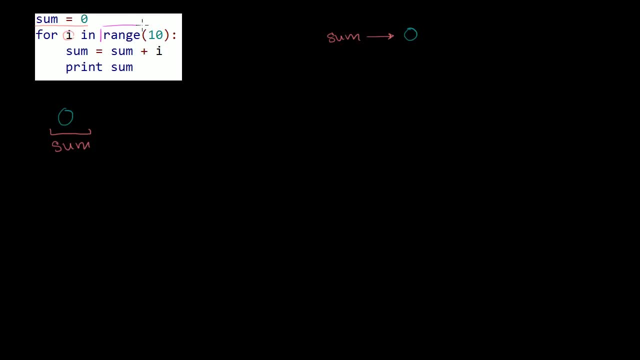 by range of 10.. So, just to be clear, if we call this right over here range of 10,, this will generate a list that looks like this. So it will generate a list: 0,, 1,, 2,, 3,, 4,, 5,, 6,, 7,, 8, and 9, up to, but not including, 10.. 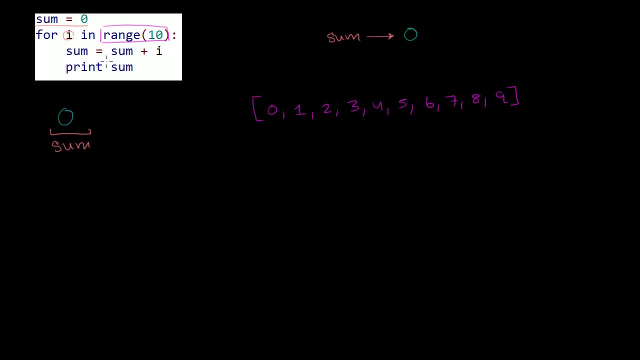 This is 10 elements right over here And then we go into the for loop. So the first time we go through the for loop- and let me write it, So I'll think about it two different ways. So one: I'll think about it in the bucket way. 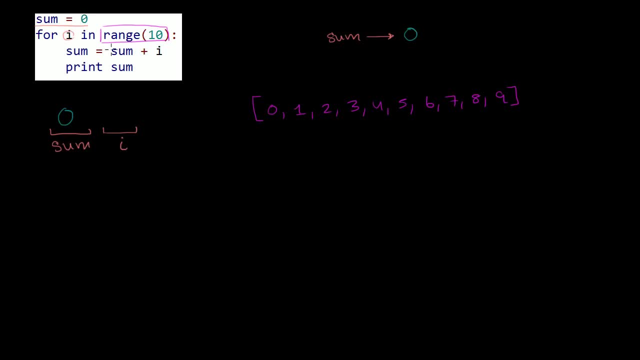 So we have this variable i that can actually only be used inside of this clause. We'll talk more about scope or where a variable could use, But this i variable is only good inside of this clause: The sum variable, the way I've defined it. 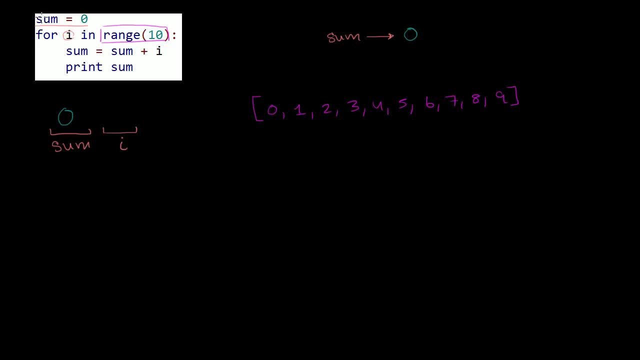 I can use it anywhere outside of the clause or inside of it, because it was defined outside of the clause, So you have your i. So this is if you think of it as a bucket, And so through the first iteration i is assigned to this first item over here. 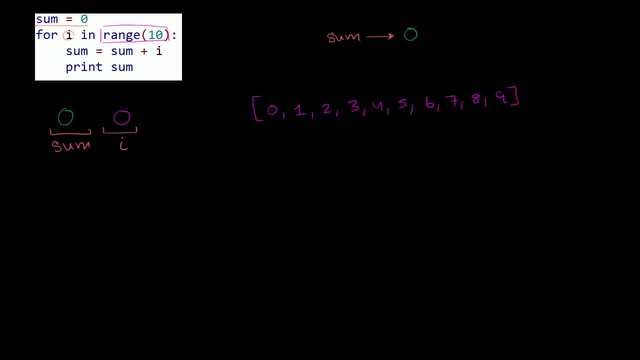 So i is going to be 0.. The reality, the better way to think about it is. i is actually referring to this first element our first time through the loop. And then we go through the loop and it says sum plus i. 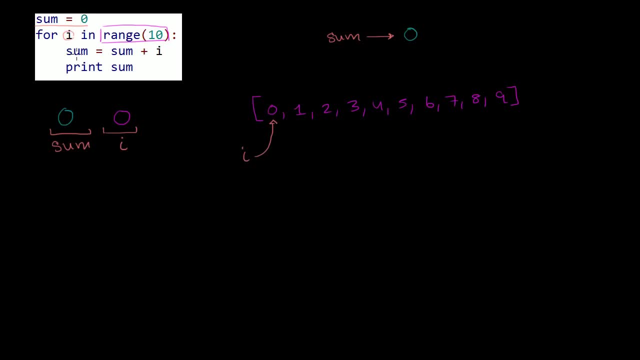 Well, sum is 0, and i is 0. You add them together, you get 0. So sum is still going to be 0, or still referring to 0. And then it prints the sum out. So then this line right over here: it prints sum. 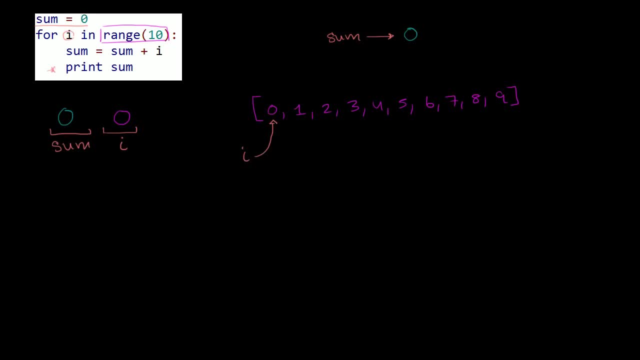 It says: OK, the sum right now is just 0, and it printed it out. Then it goes back to the for loop and says: look, are there any more elements that I can assign? i to, Well, sure, there are. 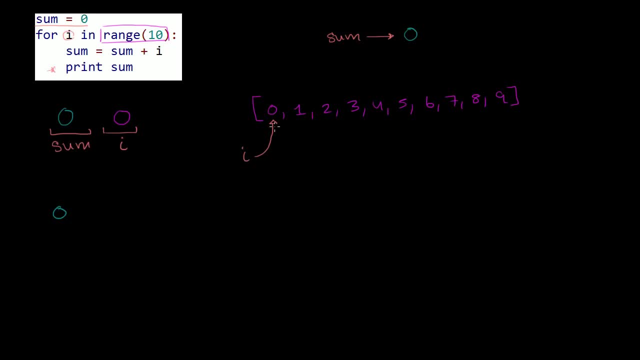 There's all of these that I have I don't have to go through. So then it makes i the next element in the sequence. So now i is going to be the next element in the sequence, Or another way to think about it, is in the i bucket. 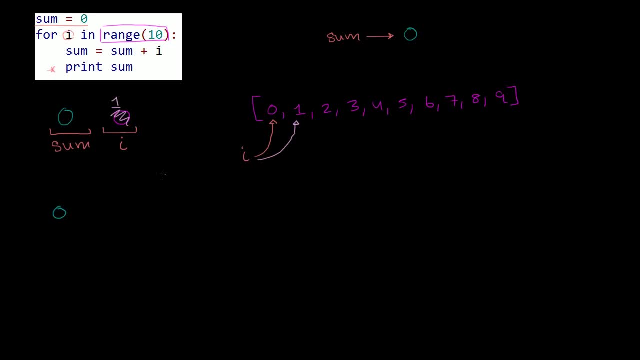 if you want to view them as buckets. i is now set equal to 1.. And now we run this again And we say, OK, sum is 0 plus i, i is 1.. So sum is now going to refer to 1.. 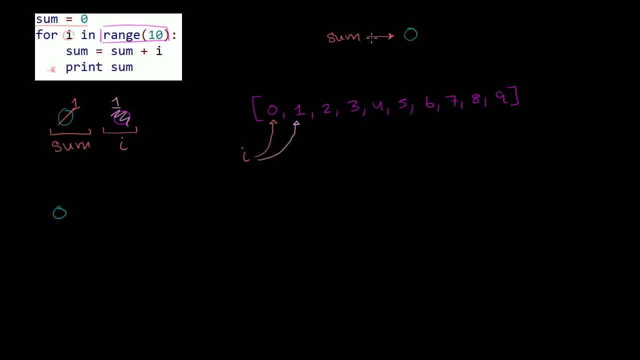 So sum is now going to refer to 1.. Or another way to think about it is: sum is now going to refer to 1.. And when you print sum, it'll now print 1.. Then the for loop will say: all right. 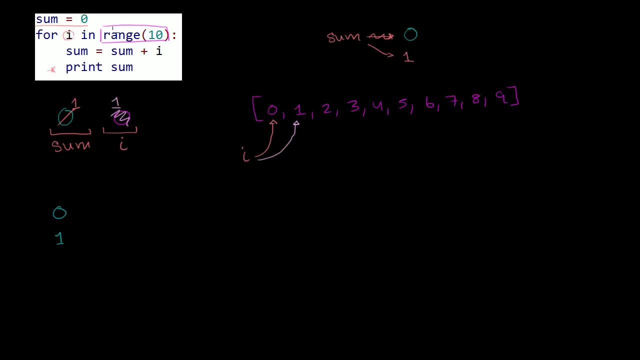 are there any more elements in this list right over here to assign i to? Well, sure, there are. There's all of these others, So let me keep going. So i can now be equal to, or can refer to, 2.. So if you think of it as a bucket, i is now 2.. 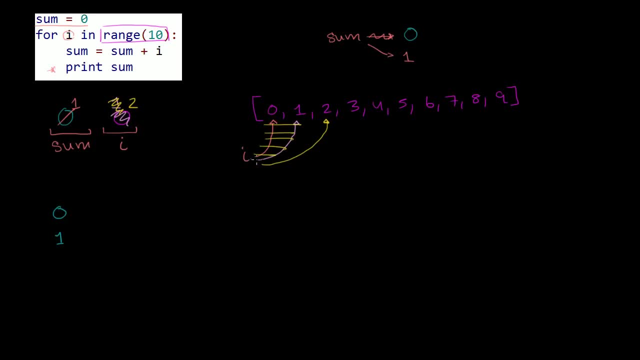 Or you can say i is now referring to 2. And you can ignore these right over here And we go through the loop again. Sum is now 1.. 1 plus i- i is now 2.. 1 plus 2 is 3..